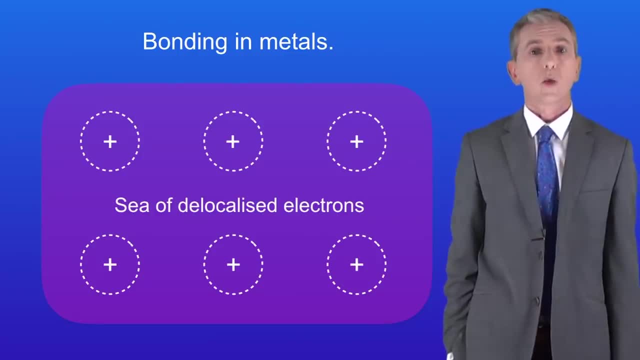 Now, because each metal atom has lost its outer electrons, we now refer to them as metal ions, But remember that this is not ionic bonding. this is metallic bonding. So the key fact is that we have a strong electrostatic attraction between the sea of delocalized electrons and the metal. 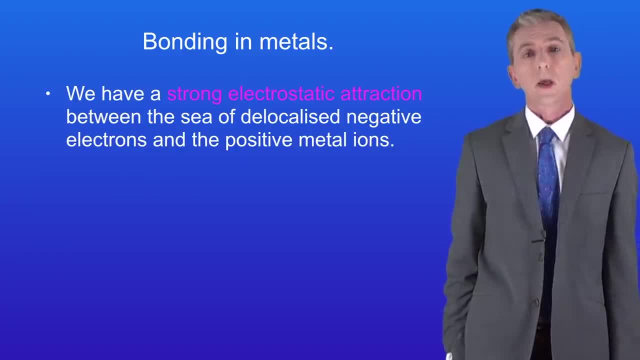 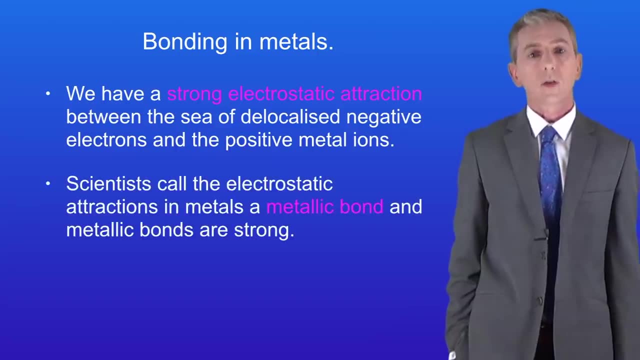 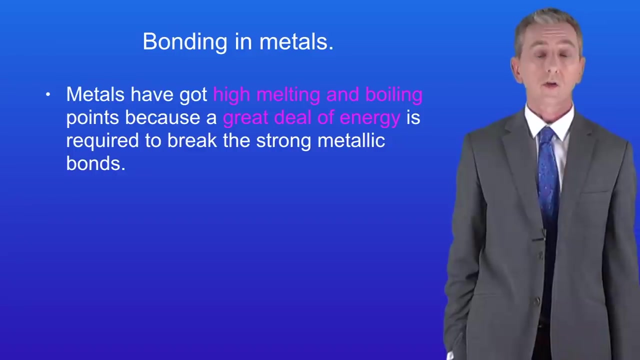 ions. Remember that an electrostatic attraction is an attraction between a positive object and a negative object. Scientists call the electrostatic attractions in metals a metallic bond, and metallic bonds are strong. Now, the strong metallic bonds explains one of the properties of metals, and that is that metals have got high melting and boiling points. That's because a great 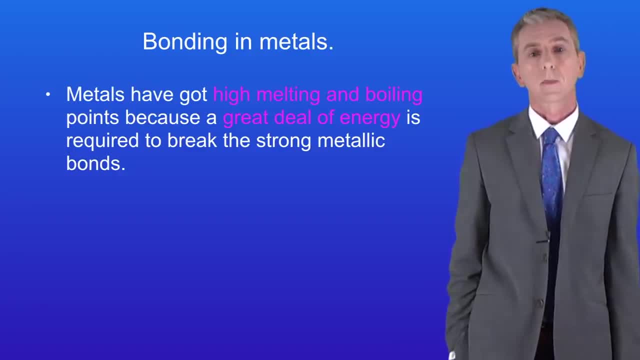 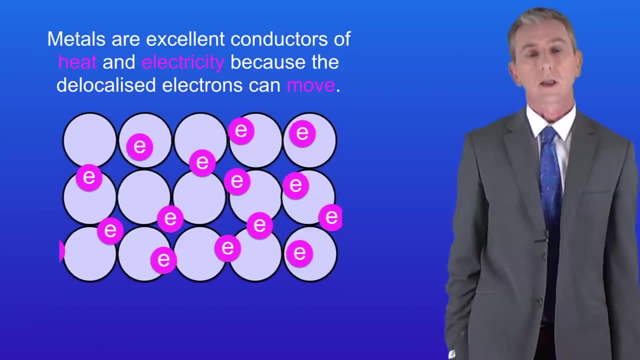 deal of energy is required to break the strong metallic bonds. The delocalized electrons are also explained another property of metals. Metals are excellent conductors of heat and electricity. That's because the delocalized electrons can move. Because electrons are charged, these moving 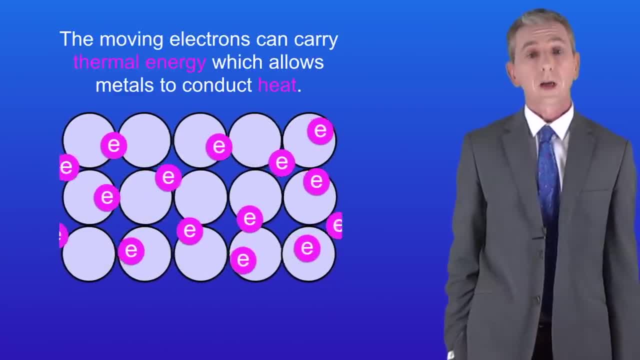 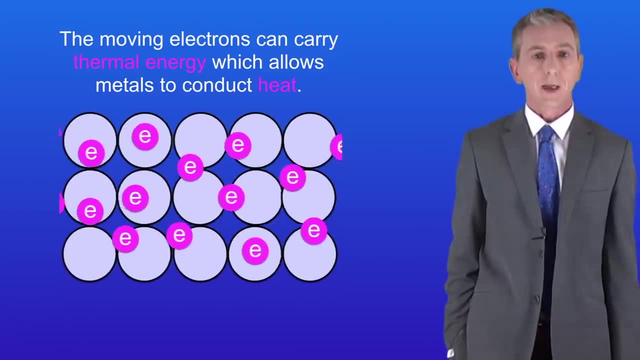 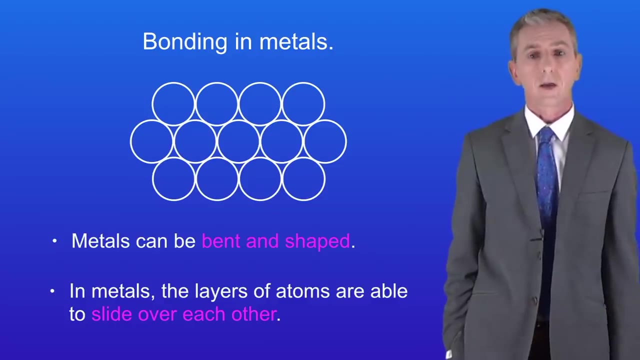 electrons can carry an electric current. Also, the moving electrons can carry thermal energy, which allows metals to conduct heat. Let's look at another property of metals: Metals can be bent and shaped. That's because in metals the layers of atoms are able to slide over each other like this: 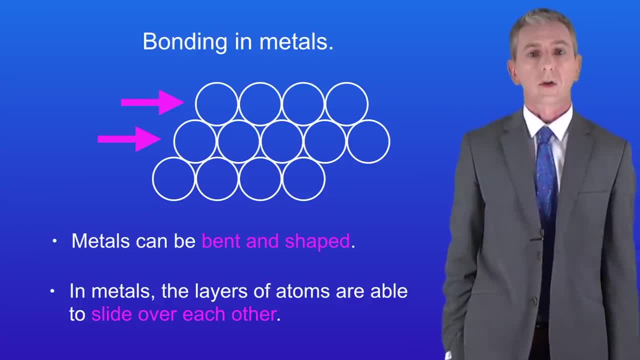 You really need to learn this, as it's a key property of metals. So, just to recap, metals can be bent and shaped, and that's because the layers of atoms can slide over each other. Now, this does give us a problem. Some pure metals just aren't hard enough to be useful. 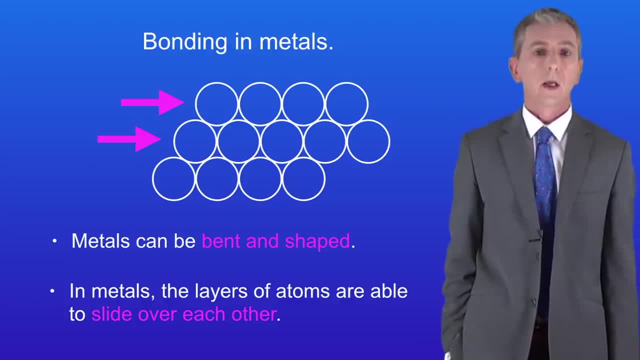 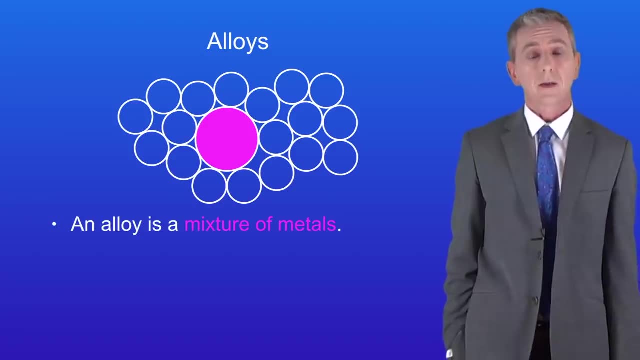 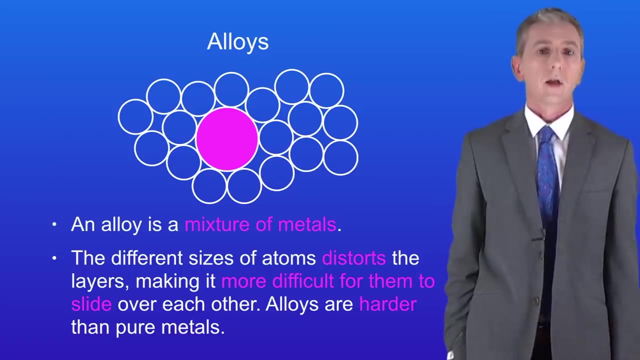 This includes copper, gold, iron and aluminium. So we need to make these metals harder and to do that, we make an alloy. An alloy is a mixture of metals. The different sizes of atoms distort the layers, making it more difficult for them to slide over each other. This means that alloys are harder. 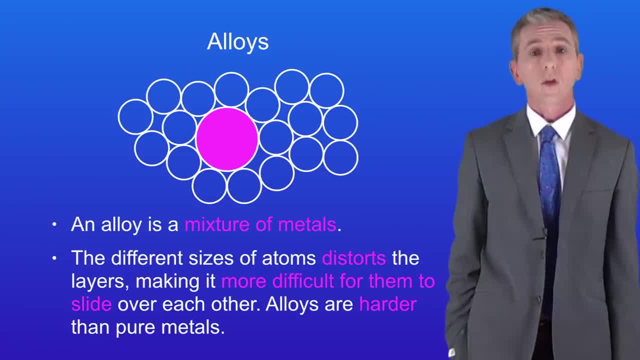 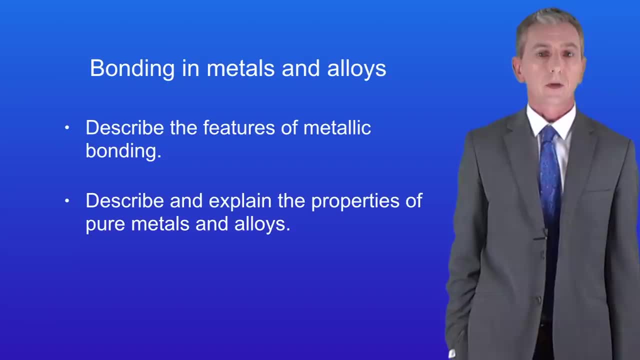 than pure metals. You'll find plenty of questions on metals and alloys in my revision workbook, which you can get by clicking on the link above. Okay, so hopefully now you should be able to describe the features of metallic bonding. You should then be able to describe and explain the properties of 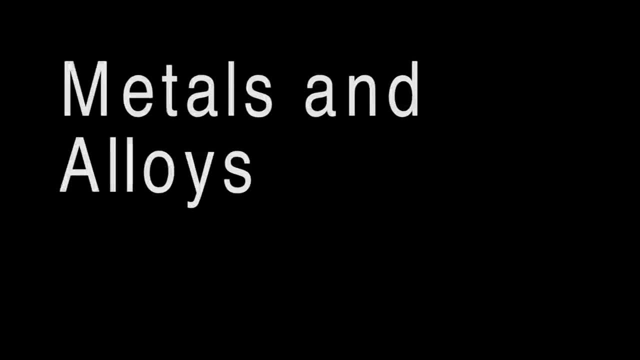 pure metals and of alloys. Thanks for watching.